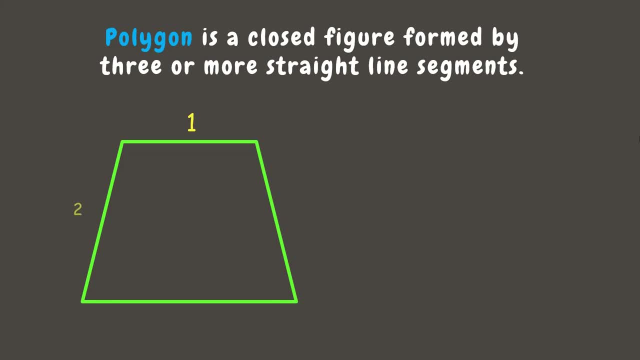 For example, this figure has one, two, three and four sides, or line segments. Line segments are straight lines. that has two endpoints. Let's name the endpoints as A, B, C and D. This means that this polygon has line segments AB, BD, CD. 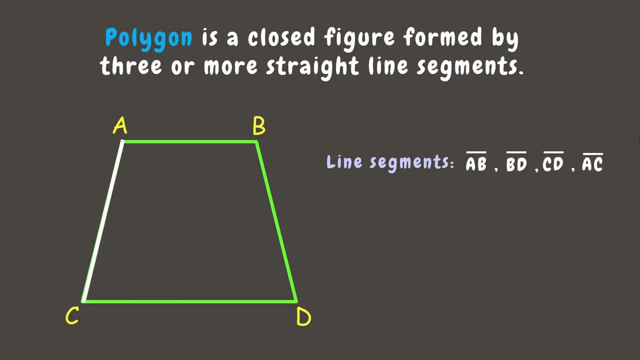 and AC, which can also be called as the sides of the polygon. Now, when two line segments meet at a certain point, they form an angle. Here this polygon has angle A, angle B, angle C and angle D, And the points where line segments meet are called vertices. 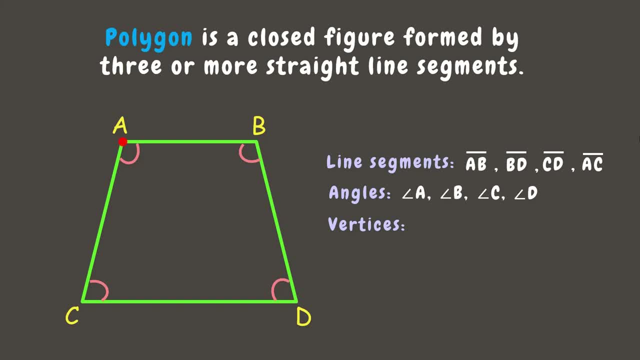 In this polygon. it has vertex A, vertex B and vertex C and vertex D. Now let's take a look at these two figures. Can you tell me which one is a polygon and which one is not? Well, the first figure is not a polygon, since it is an open figure. 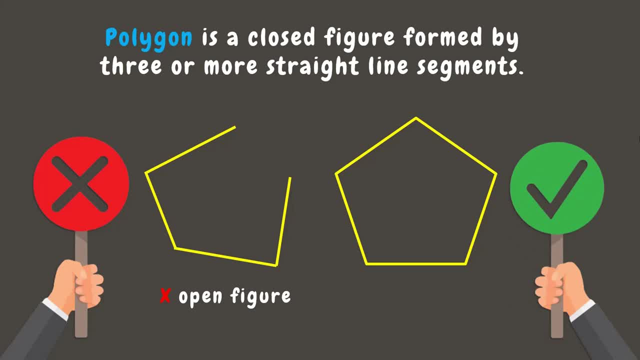 While the second one is a polygon, since it is a closed figure with straight line segments. Let's have another one. Which one do you think is a polygon And which one is not? The first figure is not a polygon, since it has curved line segments. 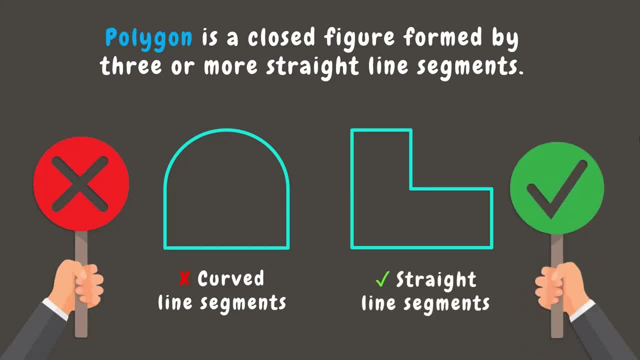 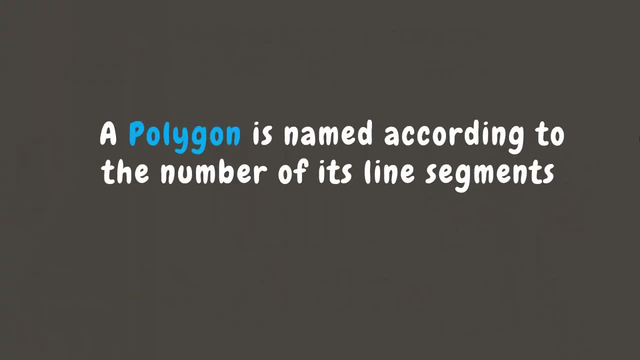 While the second one is a polygon, since it is a closed figure with straight line segments. Now, remember that the polygon is named according to the number of its sides or line segments. Now let's explore the objects that we saw in the living room earlier. 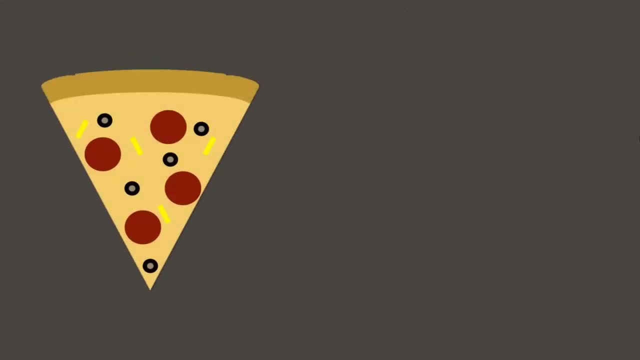 First up, we have here a piece of pizza And it has three sides, or three line segments, And this polygon is called triangle. A triangle has three sides and three angles. Here are other examples of triangles. Next one: We have here a drawer. 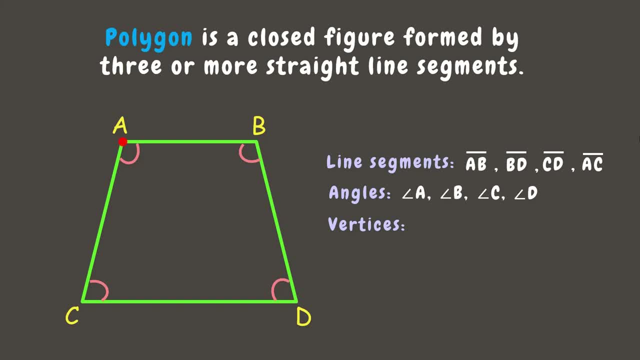 In this polygon. it has vertex A, vertex B and vertex C and vertex D. Now let's take a look at these two figures. Can you tell me which one is a polygon and which one is not? Well, the first figure is not a polygon, since it is an open figure. 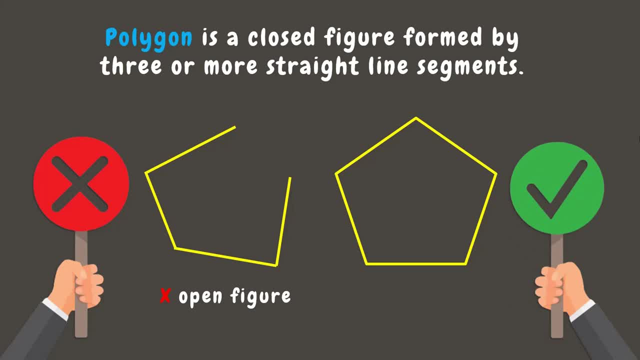 While the second one is a polygon, since it is a closed figure with straight line segments. Let's have another one. Which one do you think is a polygon And which one is not? The first figure is not a polygon, since it has curved line segments. 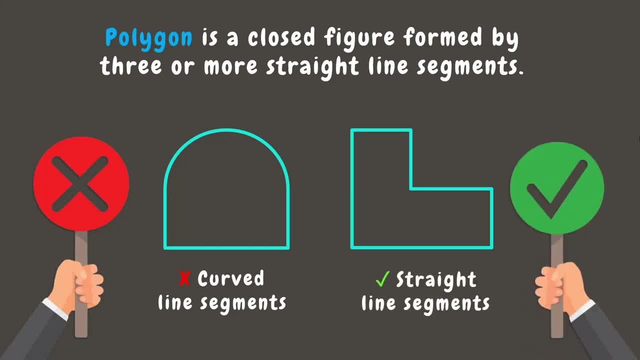 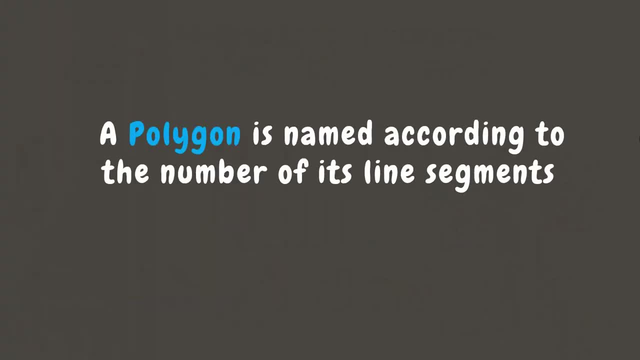 While the second one is a polygon, since it is a closed figure with straight line segments. Now, remember that the polygon is named according to the number of its sides or line segments. Now let's explore the objects that we saw in the living room earlier. 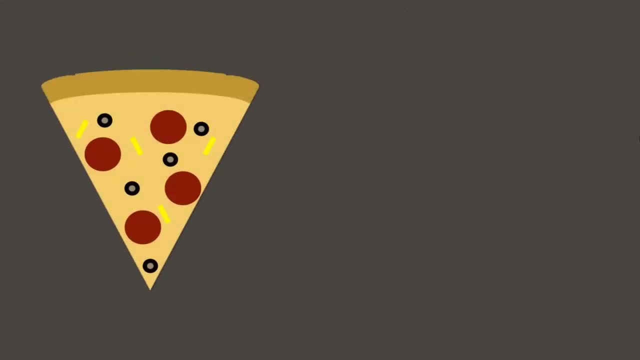 First up, we have here a piece of pizza And it has three sides, or three line segments, And this polygon is called triangle. A triangle has three sides and three angles. Here are other examples of triangles. Next one: We have here a drawer. 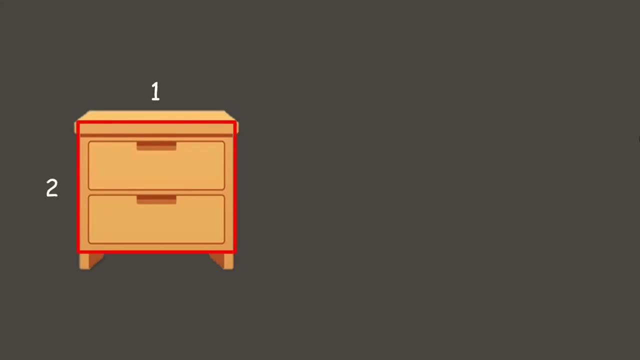 This object forms a polygon with four sides And it is called a quadrilateral. A quadrilateral has four sides and four angles. Here are other examples of quadrilateral. Other quadrilaterals are square, rectangle, parallelogram, rhombus, trapezoid and many more. 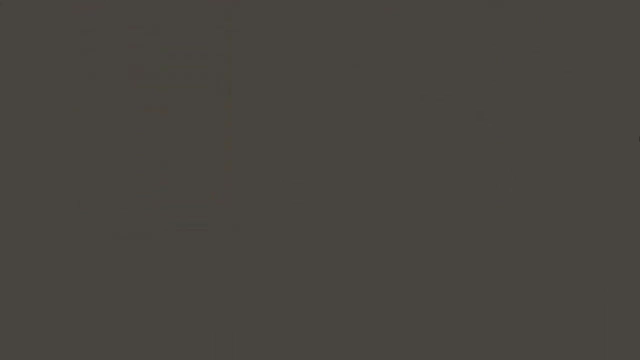 Let's go to the next one. We have a diamond. We can form a five-sided polygon from this diamond And we call this as pentagon. A pentagon has five sides and five angles. Here are other examples of pentagon. Let's go to the next one. 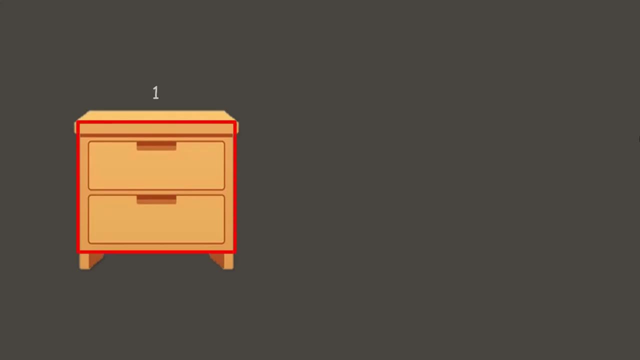 This object forms a polygon with four sides And it is called a quadrilateral. A quadrilateral has four sides and four angles. Here are other examples of quadrilateral. Other quadrilaterals are square, rectangle, parallelogram, rhombus, trapezoid and many more. 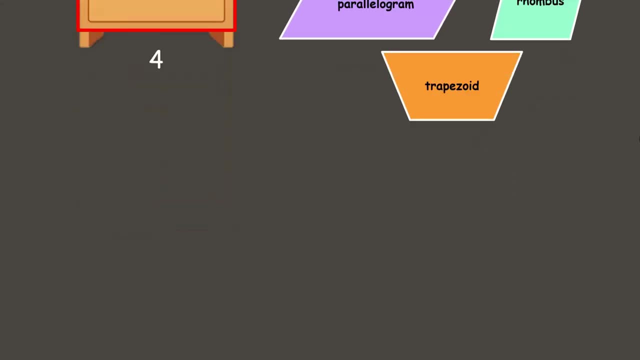 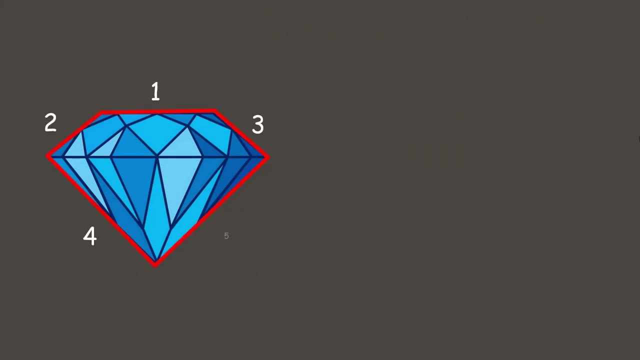 Let's go to the next one. We have a diamond. We can form a five-sided polygon from this diamond And we call this as pentagon. A pentagon has five sides and five angles. Here are other examples of pentagon. Let's go to the next one. 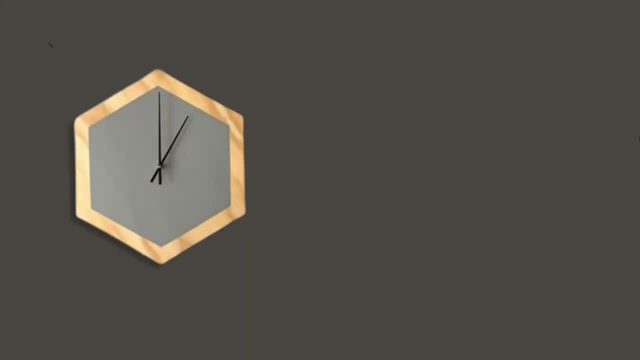 We have here a clock. This clock has six sides And a polygon with six sides is called hexagon. Hexagon is a polygon with six sides and six angles. Now here are other examples of hexagon Moving on. we have here a mirror. 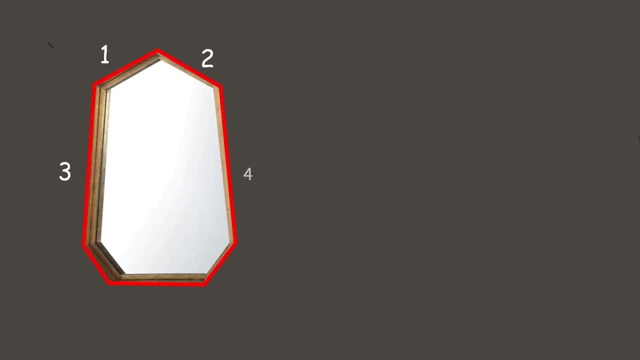 This one has seven sides, And a polygon with seven sides is called mirror Hexagon. Hexagon has seven sides and seven angles. Now here are other examples of hexagon. Perfect, Now let's go to the next one. We have a window. 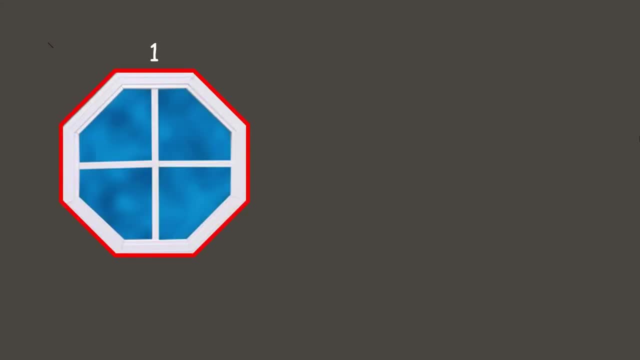 This window has eight sides, And a polygon with eight sides is called octagon. Again, octagon has eight sides and eight angles. Here are other examples of octagon. Next up, we have here a floor mat. This object has nine sides. 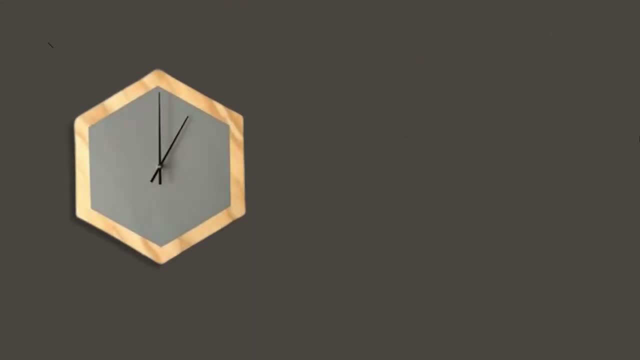 We have here a clock. This clock has six sides And a polygon with six sides is called hexagon. Hexagon is a polygon with six sides and six angles. Now here are other examples of hexagon Moving on. we have here a mirror. 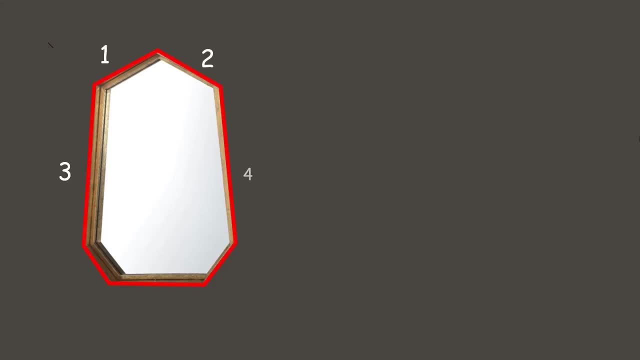 This one has seven sides, And a polygon with seven sides is called heptagon. Heptagon has seven sides and seven angles. Now here are other examples of heptagon: Perfect. Now let's go to the next one. We have a window. 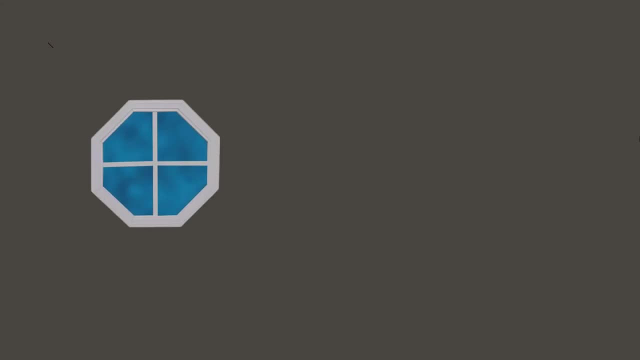 This window has eight sides, And a polygon with eight sides is called octagon, And a polygon with eight sides is called octagon, And a polygon with eight sides is called octagon. Again, octagon has eight sides and eight angles. Here are other examples of octagon. 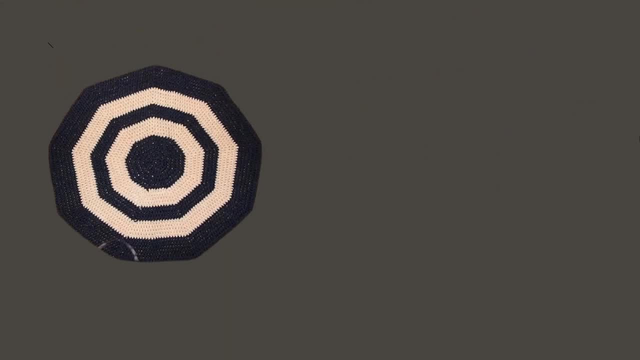 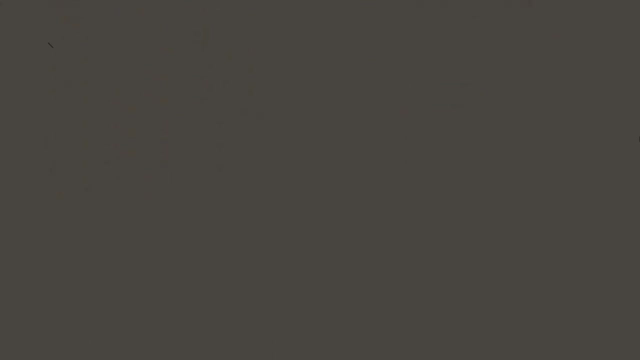 Next up we have here a floor mat. This object has nine sides, And a polygon with nine sides is called nonagon. Nonagon has nine sides and nine angles. Here are other examples of nonagon. Another object is a star. This star has ten sides. 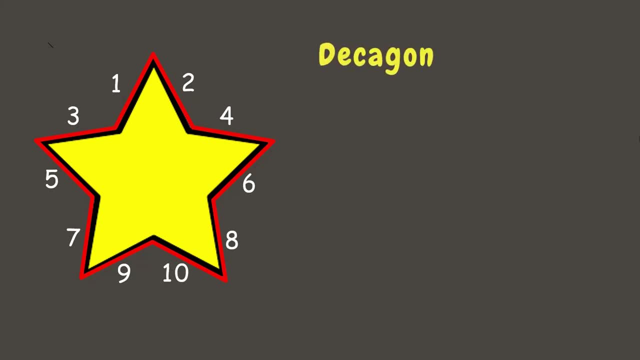 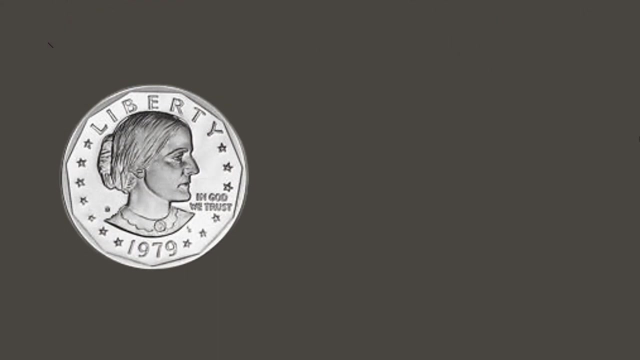 And a polygon with ten sides is called decagon. A decagon has ten sides and ten angles. Now here are other examples of decagon. Next one: we have here a coin. This coin has eleven sides. Let's count. There you go. 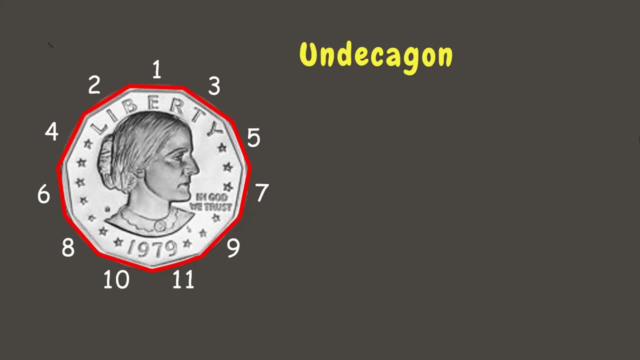 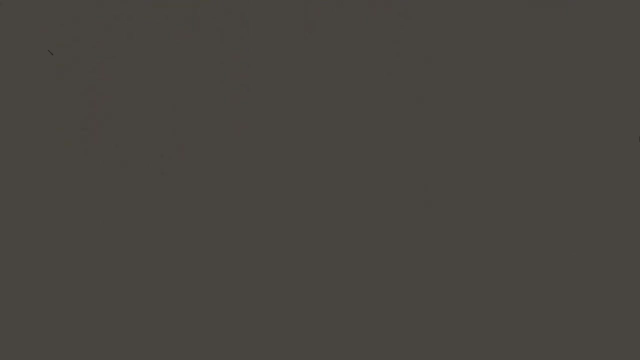 Now a polygon with eleven sides is called undecagon. Undecagon has eleven sides and eleven angles. Now here are other examples of polygons: One, Two, Three, Four, Five, Six, Seven, Eight, And a second one, a polygon with twelve sides and twelve angles.